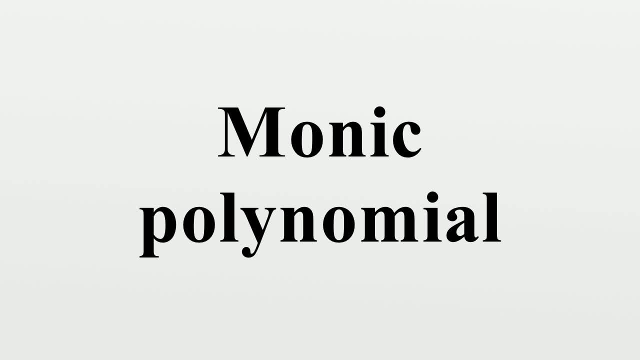 if the ring contains other invertible elements than 1.. Polynomial equation solutions. In other respects, the properties of monic polynomials and of their corresponding monic polynomial equations depend crucially on the coefficient ring a. If a is a field, then every non-zero polynomial p has exactly one associated monic polynomial q. 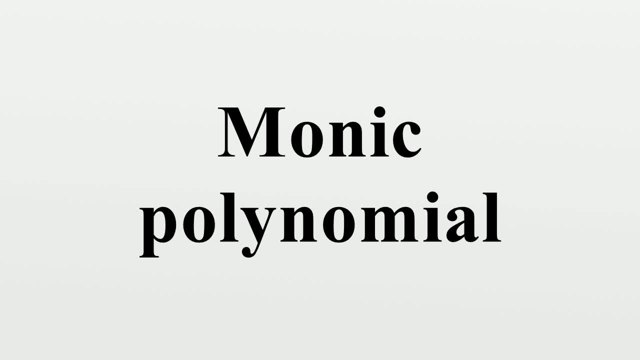 Actually q is p divided with its leading coefficient. In this manner, then, any non-trivial polynomial equation p q equals 0 may be replaced by an equivalent monic equation q equals 0.. eg the general real second-degree equation. 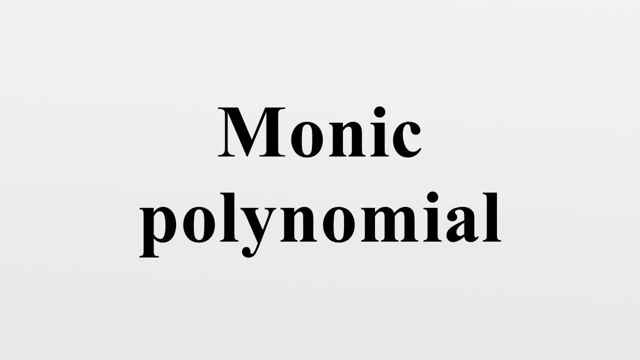 may be replaced by: by putting p equals b a and q equals c a. Thus the equation is equivalent to the monic equation. the general quadratic solution formula is then the slightly more simplified form of integrality. On the other hand, if the coefficient ring is not a field, 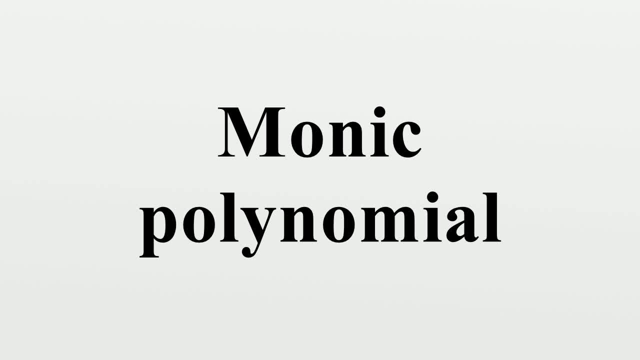 there are more essential differences, eg a monic polynomial equation with integer coefficients cannot have other rational solutions than integer solutions. Thus the equation possibly might have some rational root which is not an integer, While the equations and only may have integer solutions or irrational solutions. 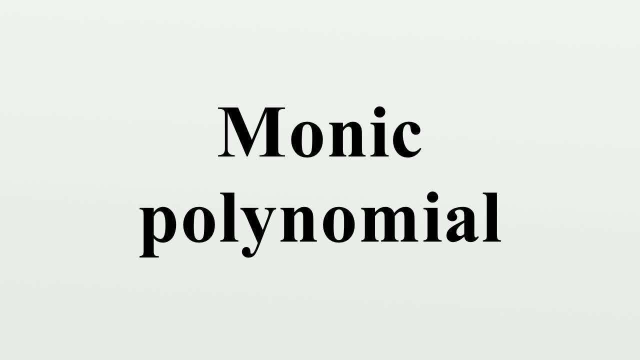 the roots of monic polynomial with integer coefficients are called algebraic integers. The solutions to monic polynomial equations over an integral equation domain are important in the theory of integral extensions and integrally closed domains and hence for algebraic number theory In general. assume that A is an. 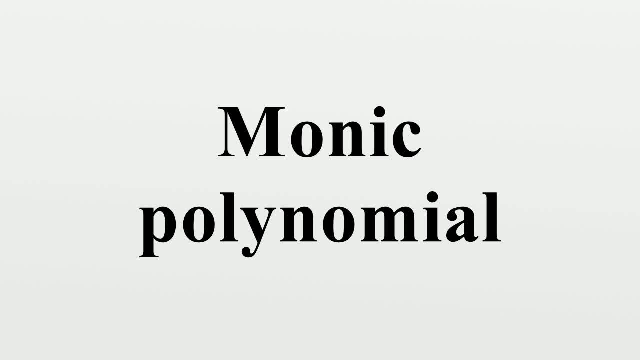 integral domain and also a subring of the integral domain, B. Consider the subset C of B consisting of those B elements which satisfy monic polynomial equations over A. The set C contains A, since any A satisfies the equation x- or equals 0.. Moreover, it is possible to prove that C is closed under addition. 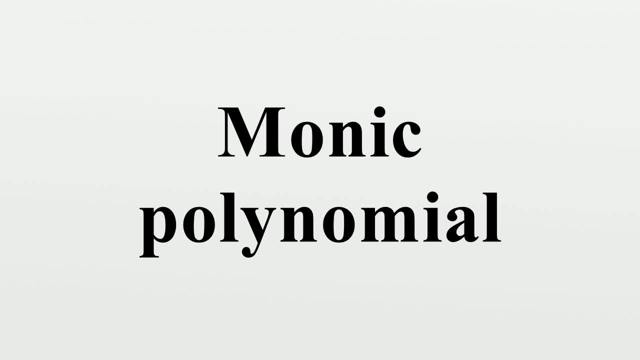 and multiplication. Thus C is a subring of B. The ring C is called the integral closure of A in B, or just the integral closure of A, If B is the fraction field of A and the elements of C are said to be integral over A. if herein, then C is.